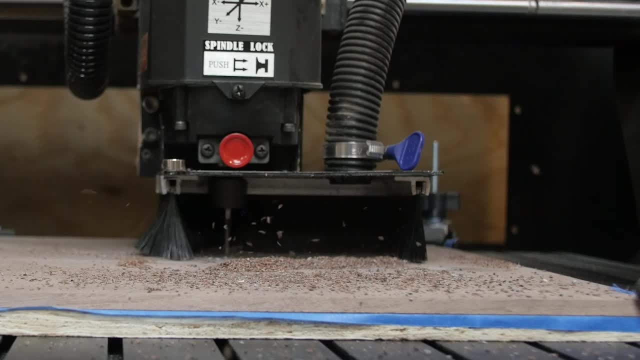 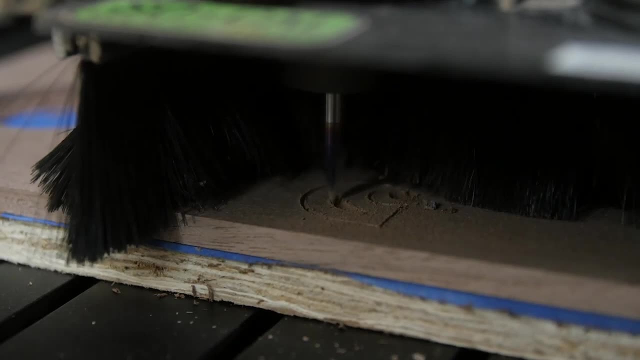 piece of wood on the CNC machine, and it'll do the work for me. I also decided to add a Carhartt branding to this, since this whole series is powered by my friends at Carhartt. so I can't thank them enough, and I thought it would be a nice touch to give this to them as a gift, for. 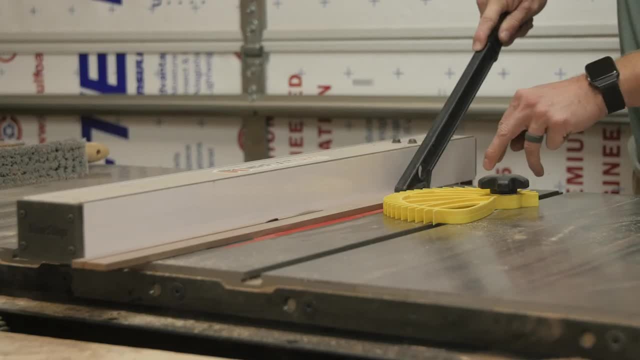 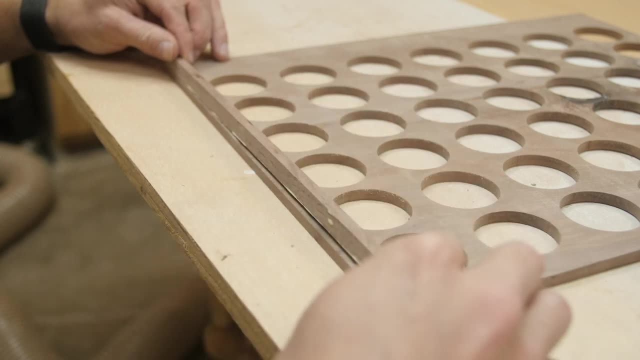 making this series possible. I'm going to strip a bunch of small strips of walnut to act as the dividers between each column. This took a little bit of trial and error to figure out what the proper size needed to be, but once I had it figured out I could cut the opposite side so that I had two halves. 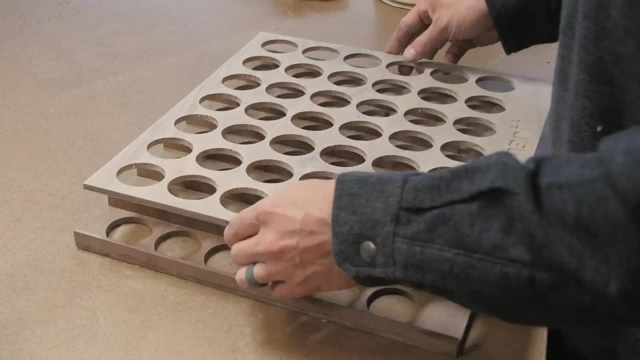 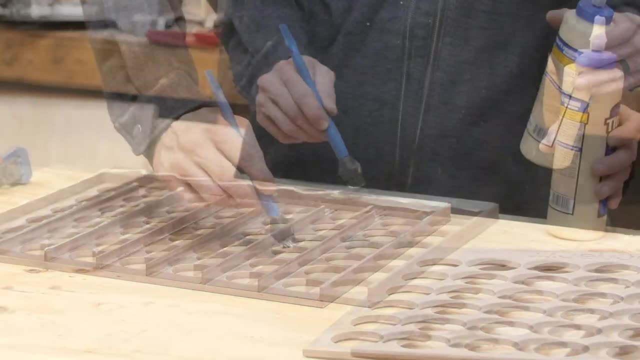 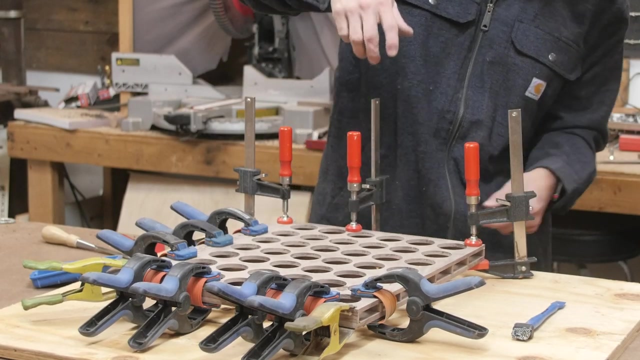 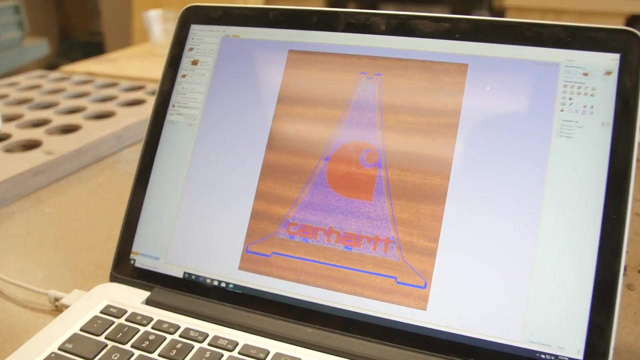 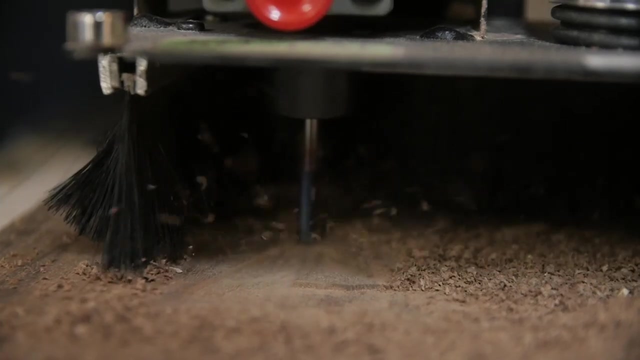 and then glue everything together. From there I can move on to starting the base. I decided to use the CNC to cut and engrave the legs for the game as well. While the legs were cutting on the CNC, I moved on to how to attach the legs to the game board. I'm using some brass dowels to attach the 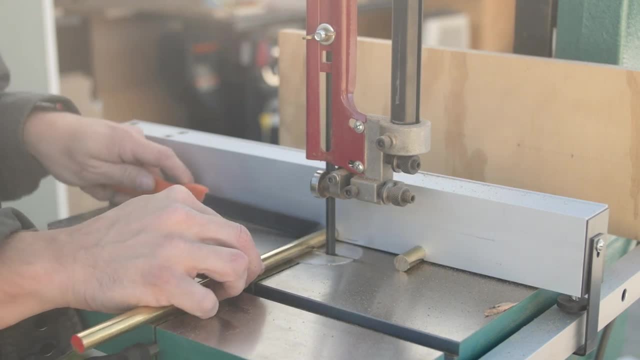 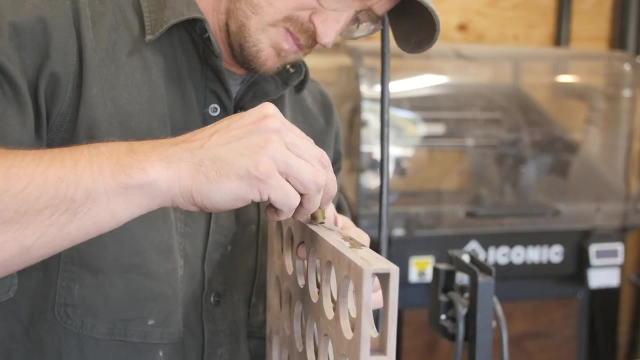 legs so the game board can swivel and tip upside down so the game pieces can dump out. So I cut a couple small pieces of the brass rod on the bandsaw, sanded them down a little bit, drilled some holes into the side of the board and glued them in place with some CA glue. 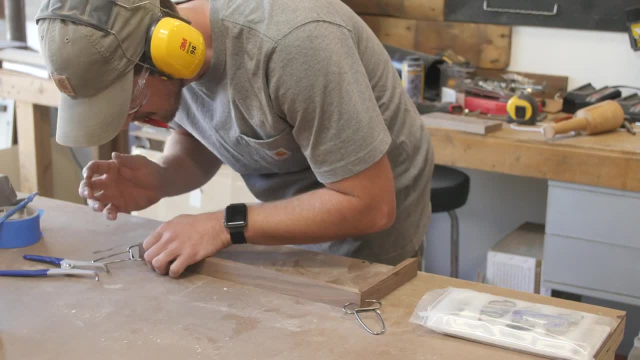 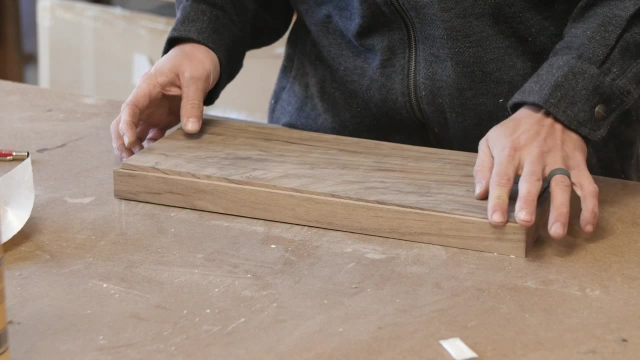 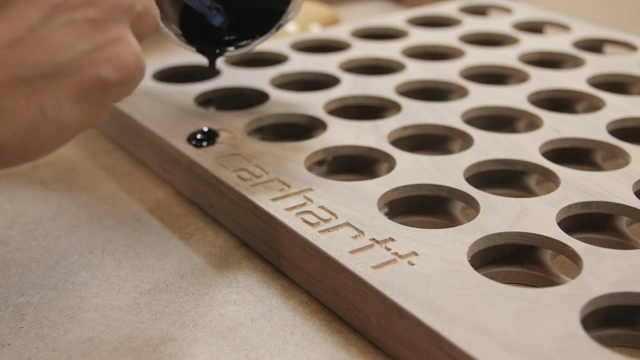 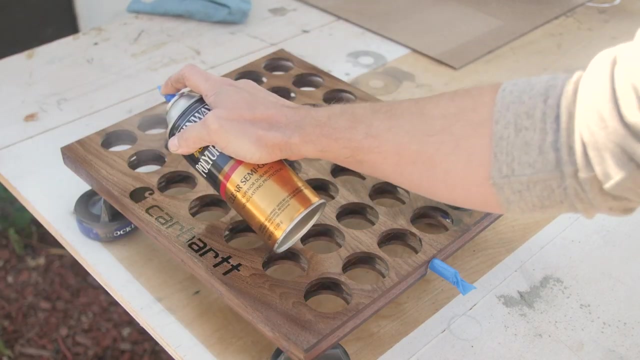 I also built a small tray to connect the two legs to make the base one solid piece and also offer a place to catch the game pieces From there. I could move on to finishing the whole game board. I added some black epoxy to fill in the CNC logos on the board, sanded everything down and added several coats of. 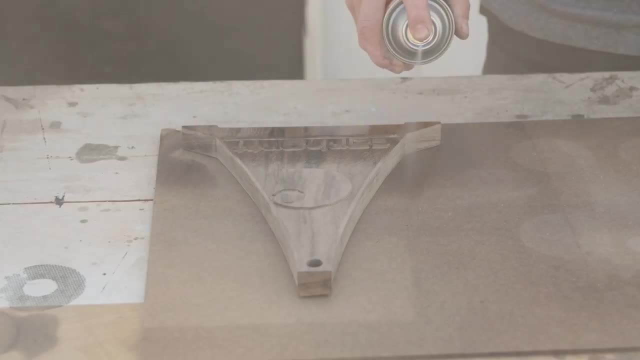 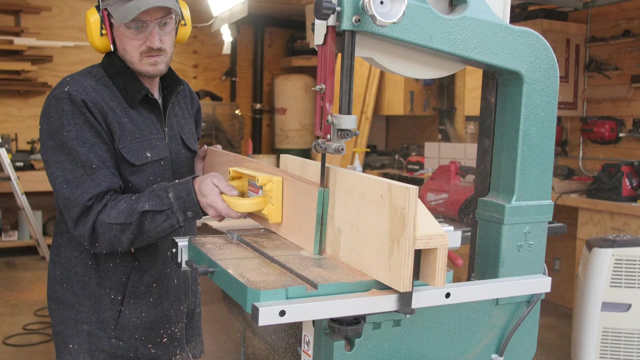 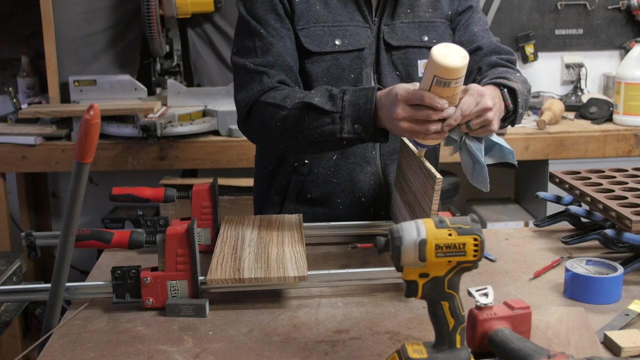 semi-gloss spray, polyurethane to finish it off. With the board complete, I moved on to making the game chips. I decided to make the chips out of some zebra wood, like the jewelry box I previously made and milled and glued up a panel. 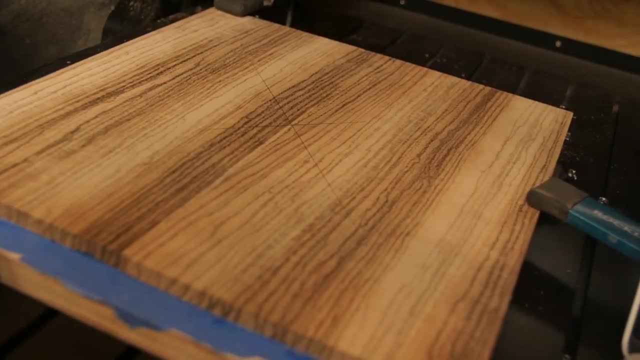 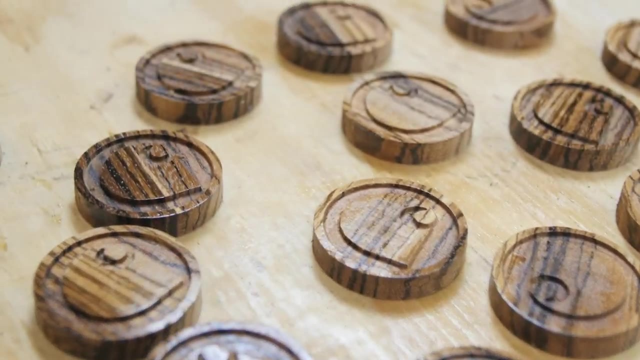 Then I designed and cut the pieces on the CNC machine. Each chip has the Carhartt logo in it. For one half of the game pieces I left it as the plain zebra wood and for the other half I filled them with black epoxy so you can differentiate between the two teams. 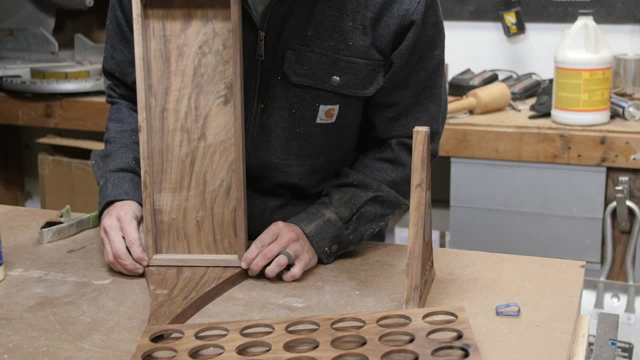 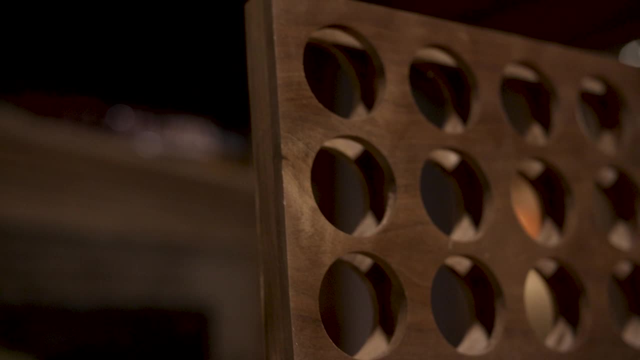 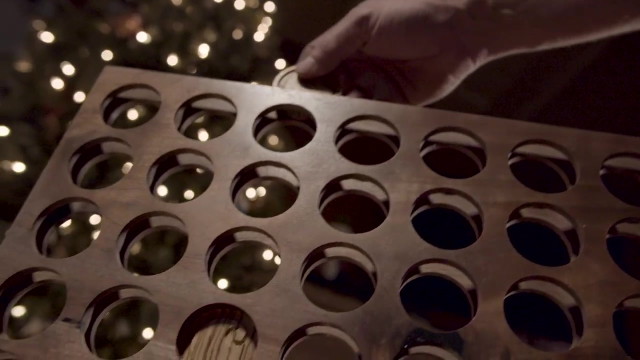 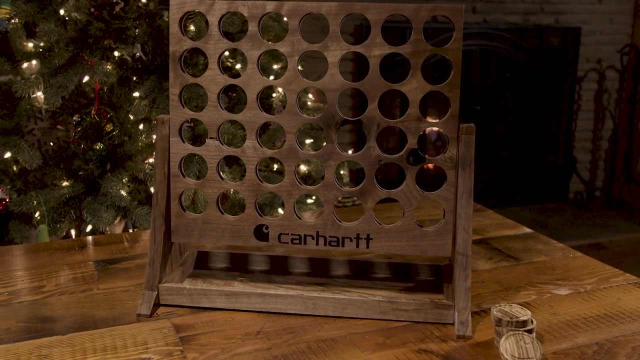 Once all of that is finished, I could assemble everything and this project was complete. So that's it for this project. I realize that it's a pretty involved project and that not everybody has access to a CNC machine like I do, but it does make things easier. Could you do it without? 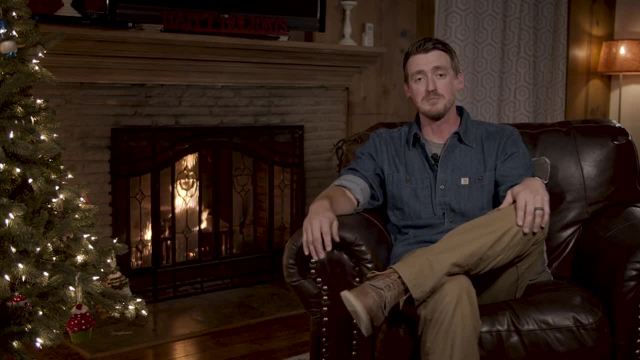 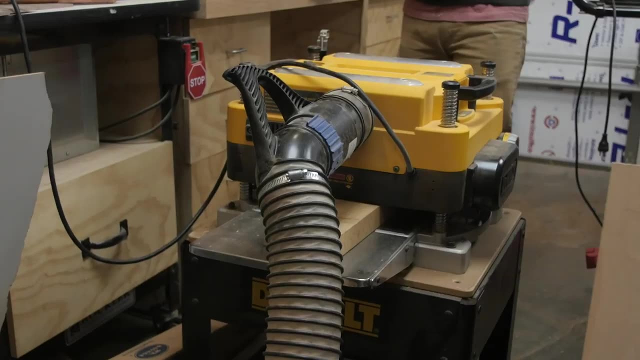 it. Sure, Could you make different versions of it without it? Probably, But I'm just showing you what's possible if you're willing to invest the time, the effort and the money into the tools. So we're not quite done yet. Next, I'm going to show you how to tackle a 3D chess board. 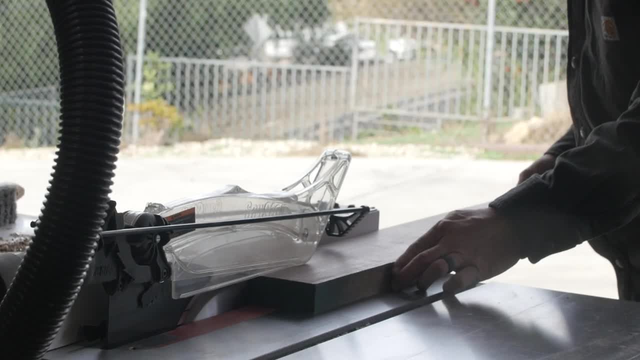 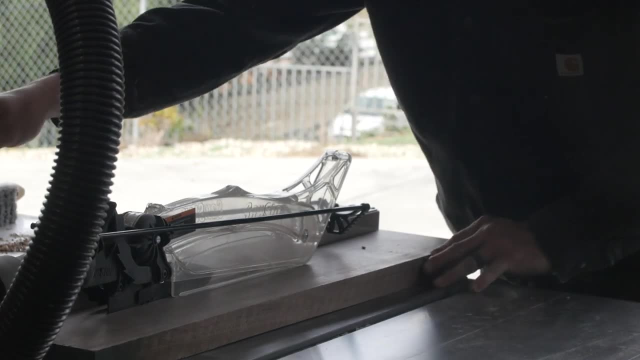 and, like most projects I've done, it involves milling some lumber down. first I'm milling some light colored maple and some dark colored walnut and ripping it on the table saw to create inch and a quarter by inch and a quarter long strips. Next I'll take it over to the chop. 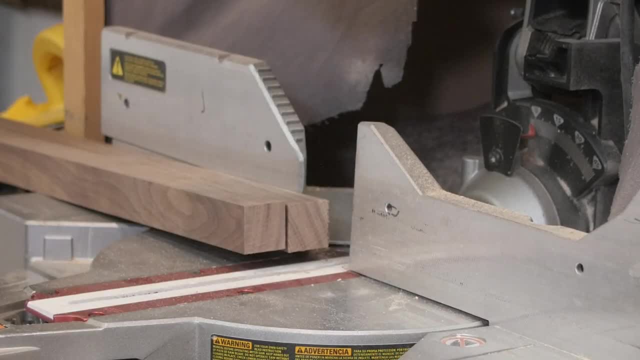 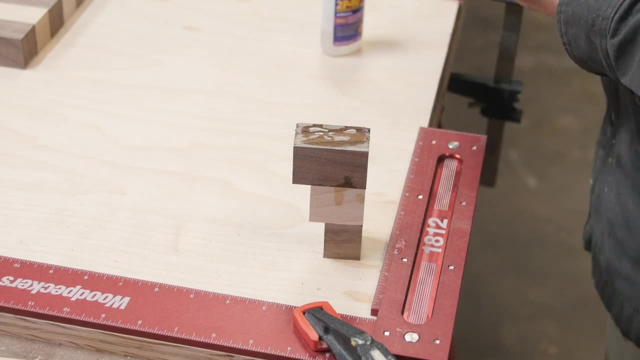 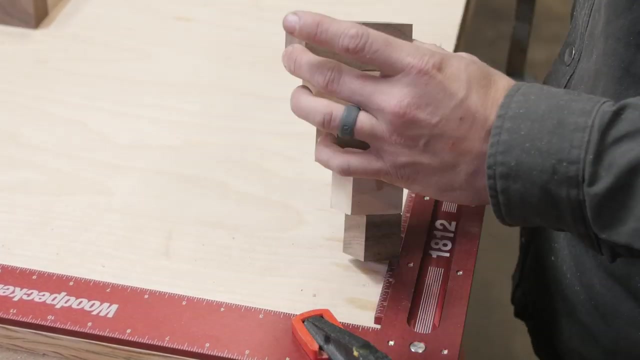 saw and cut it into a ton of small pieces at half inch increments, with the longest piece being four inches and going down from there. Once I have a bunch of pieces cut, I start gluing them up. This project just involves a lot of cuts and a lot of glue, Stepping up or down each piece by a half inch with 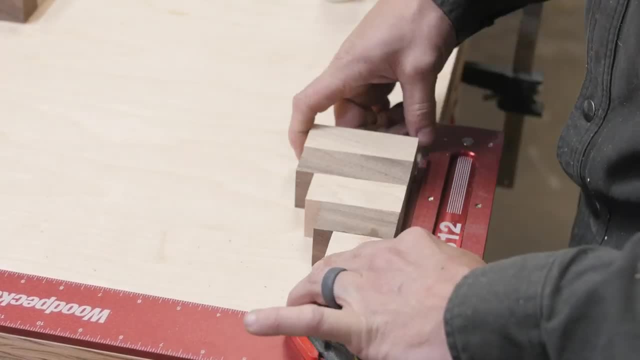 the king and queen being the tallest and everything else stepping down from there. So once I have the first row done, it is time to cut the others out. Also, I'm going to go ahead and New row done, I can do the second row, and then so on. 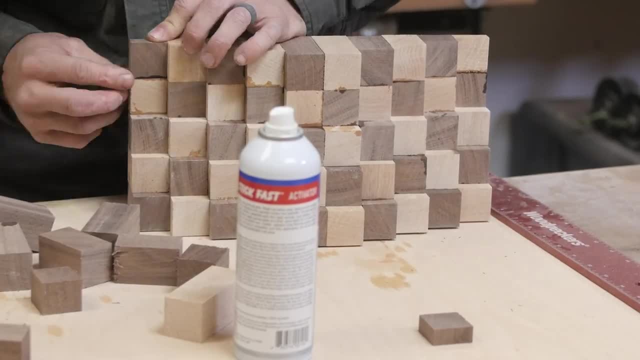 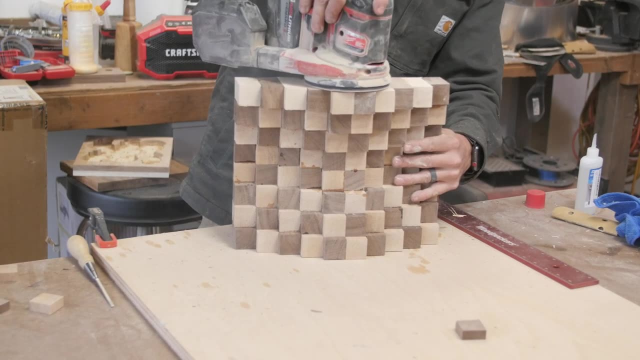 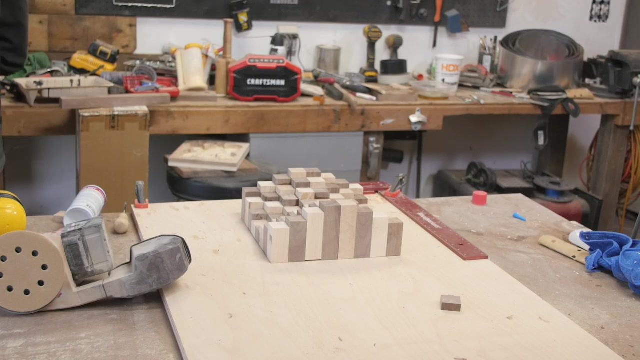 Now the board should be eight rows by eight rows, but at this point I realized I made the board eight rows by ten rows. so I took it to the table saw and ripped one row off each side to keep it eight by eight. From there I cleaned it up with the sander and then could start on making a nice